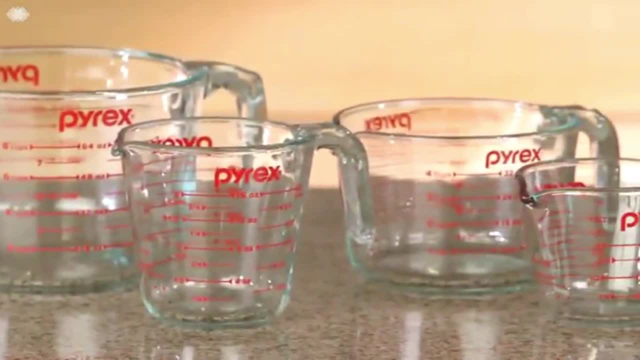 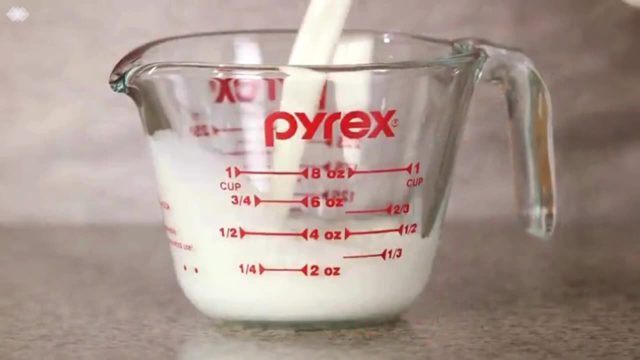 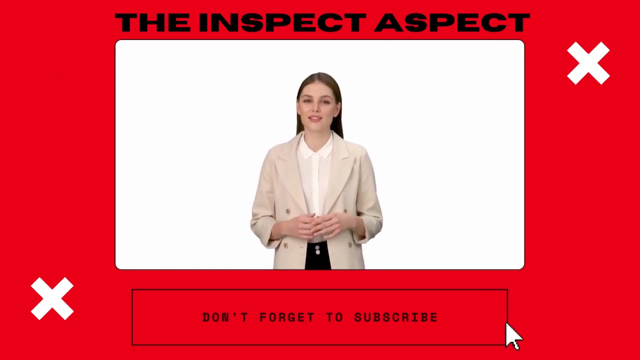 Are you looking to elevate your baking and cooking game? Discover the charm of the Pyrex 3-piece glass measuring cup set. Is it the secret ingredient to your kitchen success? Let's find out. Welcome to the Inspect Aspect, where we dive deep into products. 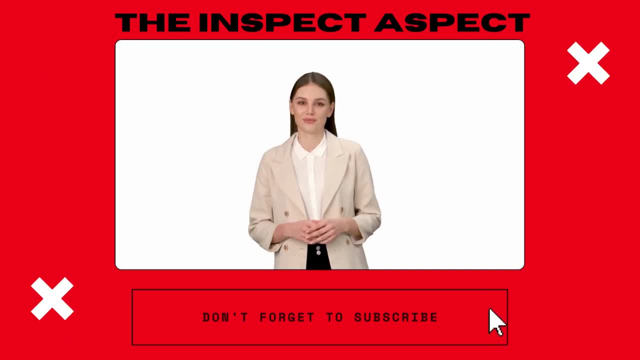 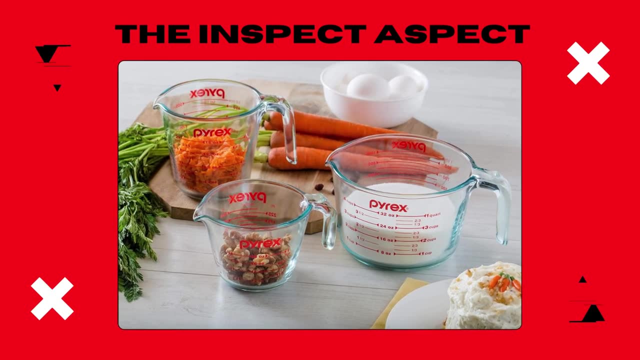 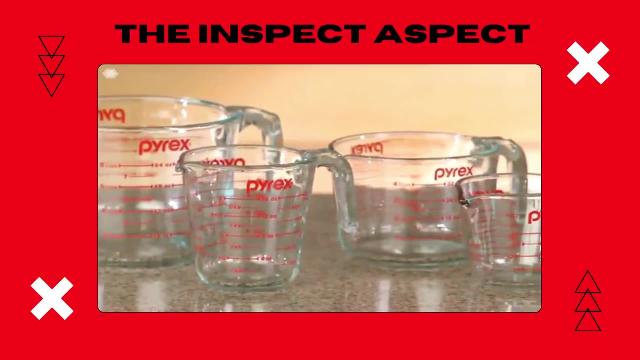 revealing pros, cons and everything in between. In today's review, we're focusing on the Pyrex measuring cups, a staple in any modern kitchen. With their elegant design and practical features, they promise to make your cooking and baking experiences even more delightful. This set's variety is perfect for every recipe from a. 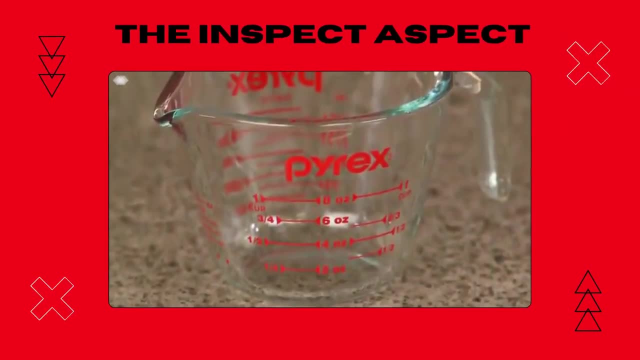 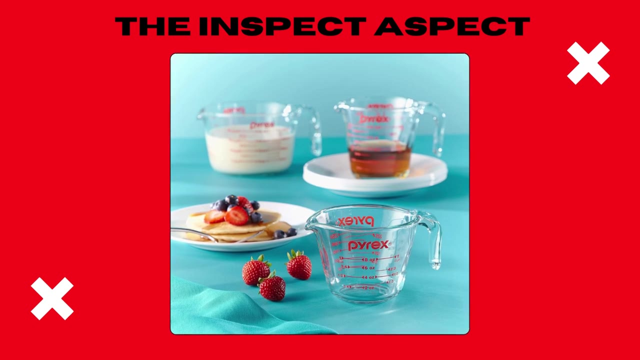 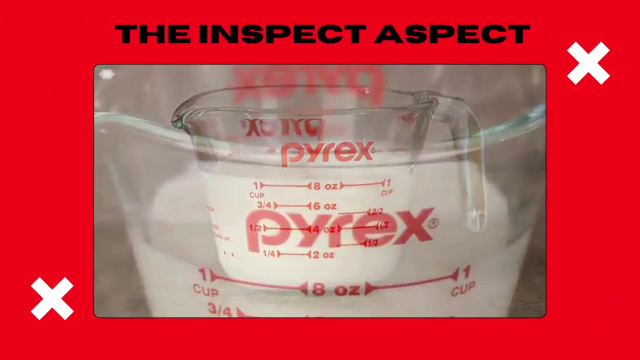 single cup of flour to a larger mix. The sizes are designed with your cooking needs in mind, making them a versatile choice for any kitchen. Clarity is crucial in perfecting recipes. These cups feature easy-to-read markings ensuring precise measurements every time. Say goodbye. 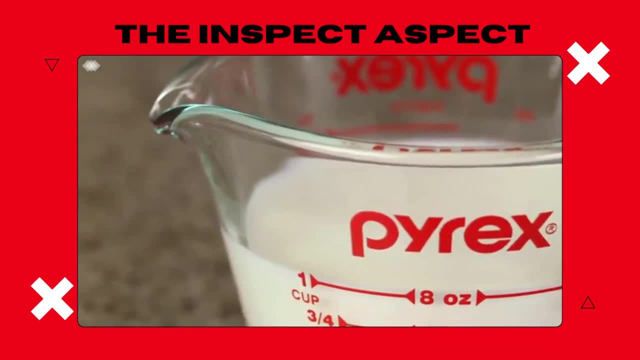 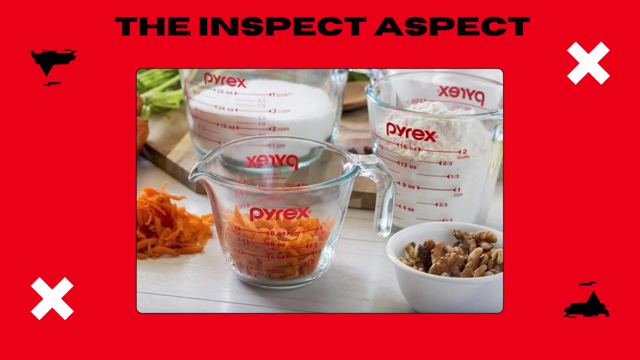 to guesswork in your baking. If you have any questions, feel free to reach out to us. Handling liquids is a breeze with their comfortable grip and spill-free spouts. Whether you're a baking enthusiast or a busy mom, these cups add convenience to your kitchen. 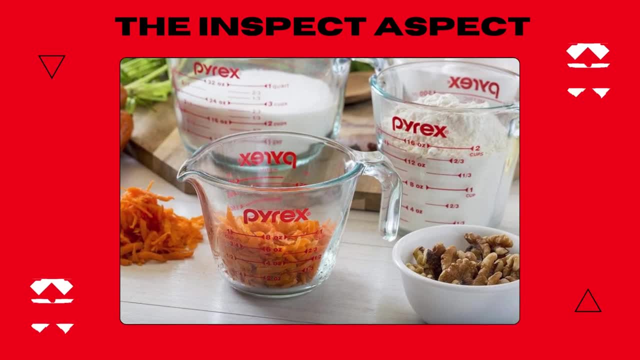 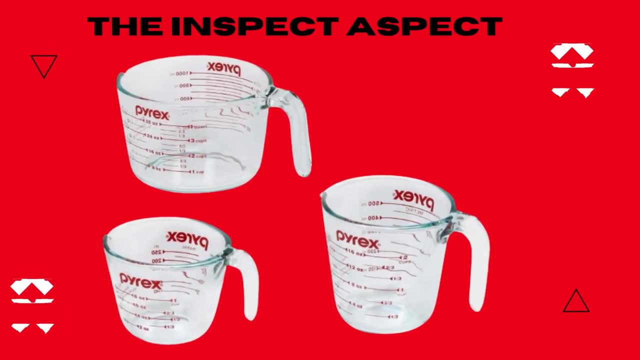 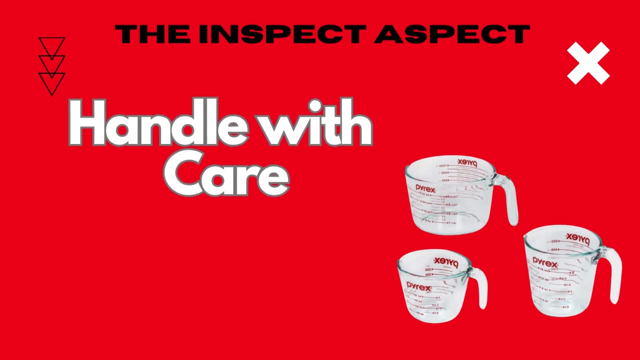 routine Safety meets style with these BPA-free, non-toxic glass cups. They're made to last, ensuring a lasting addition to your kitchen collection. However, remember they are glass and need careful handling. A gentle touch will ensure they remain a long-term companion in your 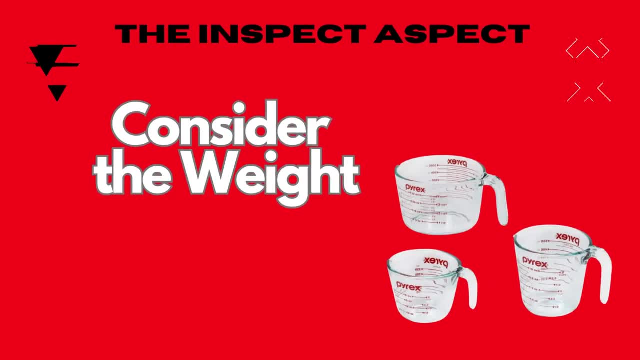 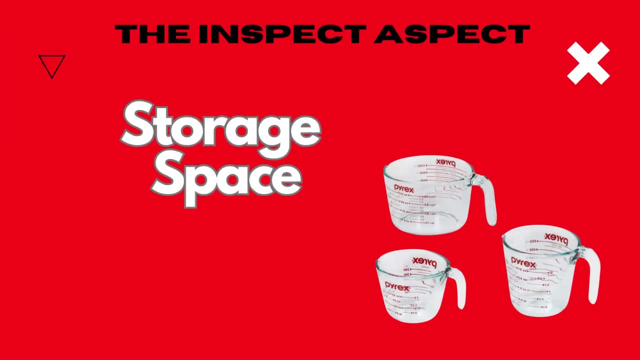 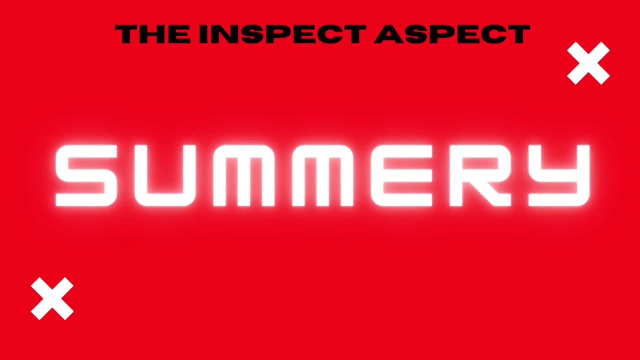 culinary adventures. They are a bit on the heavier side. If you prefer lightweight tools, keep this in mind. Lastly, they do require some storage space. A little rearrangement in your kitchen might be needed to accommodate these beauties. To wrap up, the Pyrex Glass Measuring Cup Set combines elegance with functionality, making them 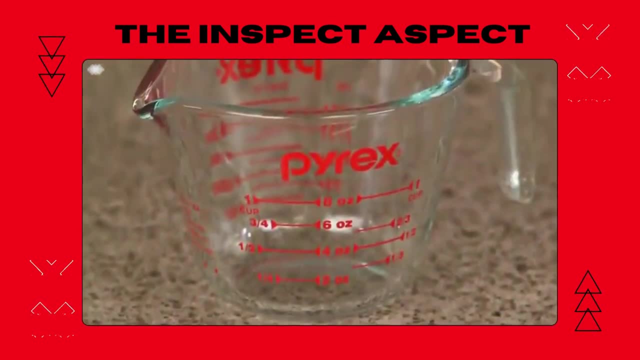 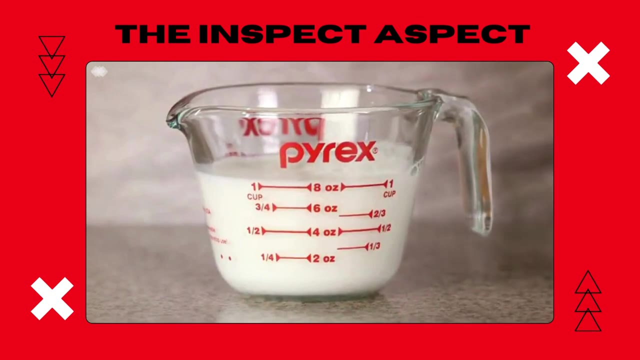 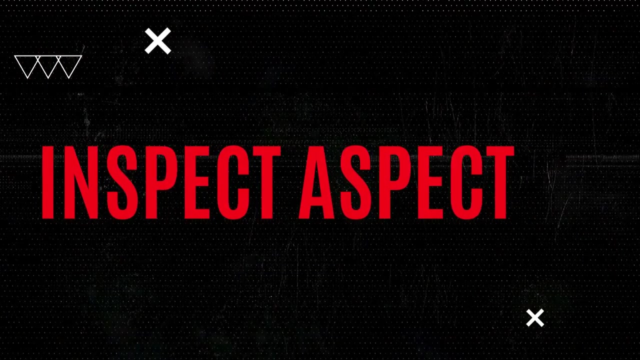 a cherished addition to any kitchen. Thanks for joining us on the Inspect Aspect. Like, comment and subscribe for more kitchen essentials tailored for you. Don't forget to check out the link in the description for more details on the products we review.